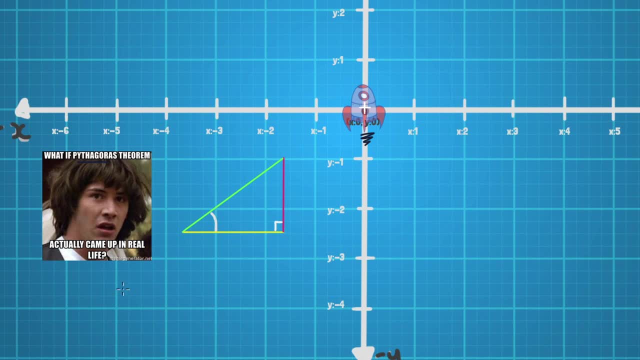 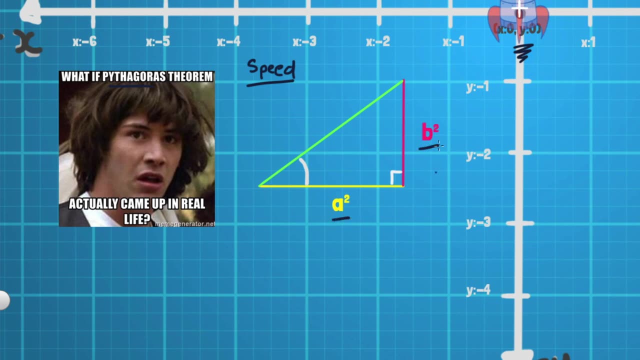 game. so games are technically not real life, but they occur in real life. so i'm claiming real life. we're going to be using pythagoras's theorem to understand speed, but firstly the theorem. so we've got a squared plus b squared is equal to c squared. you can think of this as the square of one side. 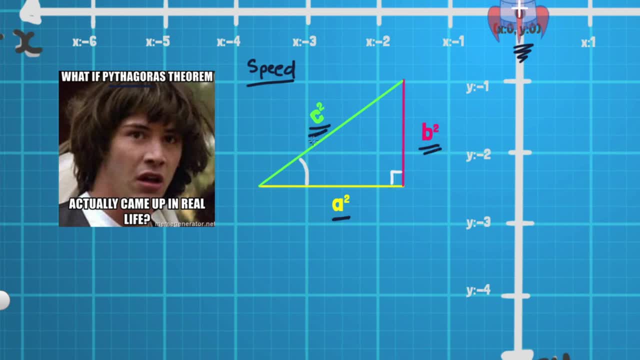 plus the square of the other side, equaling the square of the longest side of the right angle triangle. and here's our formula: a squared plus b squared is equal to c squared. now we can just substitute some values in, so we're going to go ahead and do that, and we're going to go ahead and. 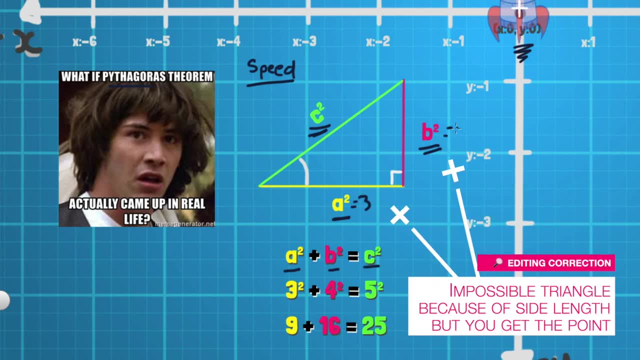 we're going to go ahead and do that, and we're going to go ahead and do that, and we're going to make a equal to three. we could make b equal to four and c would be equal to five, because three squared plus four squared is equal to five squared. three squared. well, that's just nine three times. 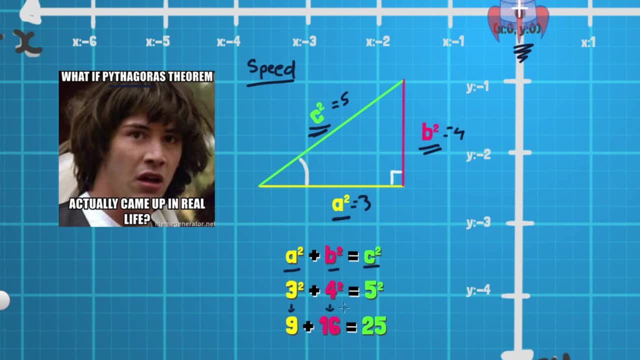 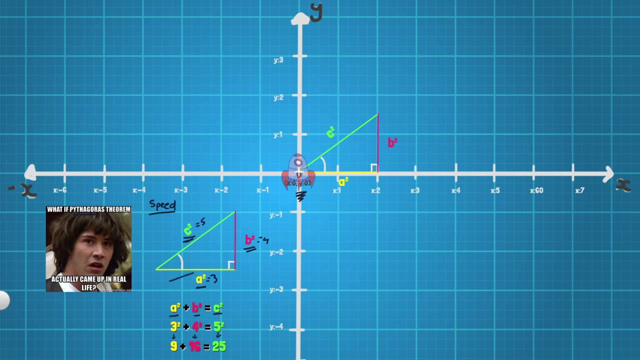 three is equal to nine. four. four times four is sixteen, so nine plus sixteen is equal to twenty five five squared. what i've done is take a copy of our right angle triangle down here and placed it directly on the ship. what this shows is, if we wanted to get our ship to this point right here. 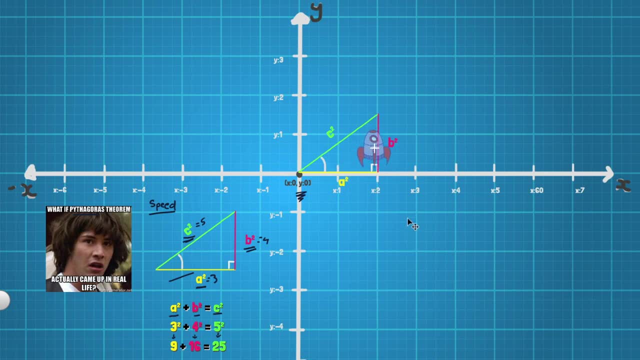 our ship would move across the x-axis here and move up the y-axis here. we can just substitute those names because, remember, the change in the x value is just the x velocity and the change in the y value is just the y velocity. if that's confusing, go check out the card in the top right hand corner and then come back to this. 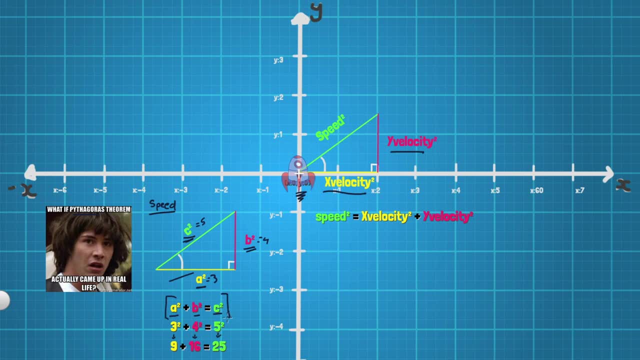 tutorial. so refer to our formula down here, where we had a squared plus b squared, is equal to c squared. well, c squared is just the speed, remember, that's the long side and that's the same thing as the a squared, which is our x velocity here, plus b squared, which is our y velocity. now, our change in. 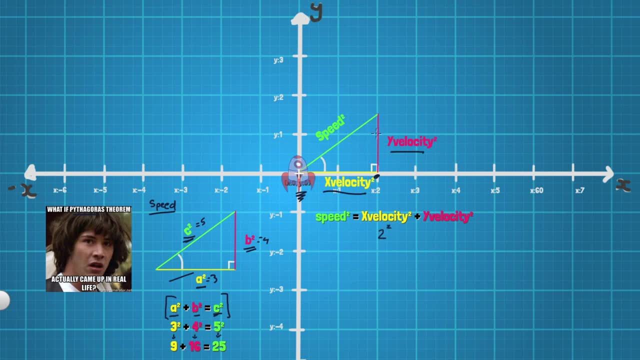 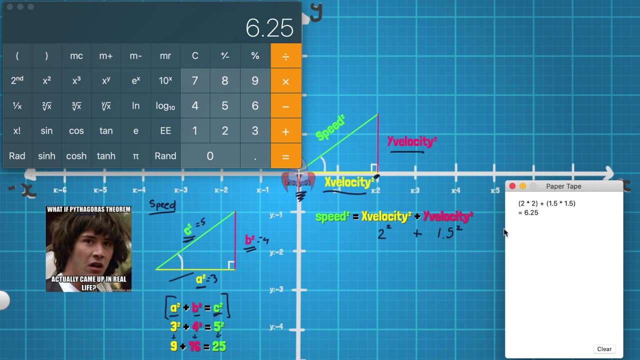 y is equal to c squared, so that would be two squared. our change in y value? well, that's around 1.5. so we go 1.5 squared here. we need to add those two things together and i just got the calculator to help us out with that. two square, so two times two plus one point. five times one. point five is: 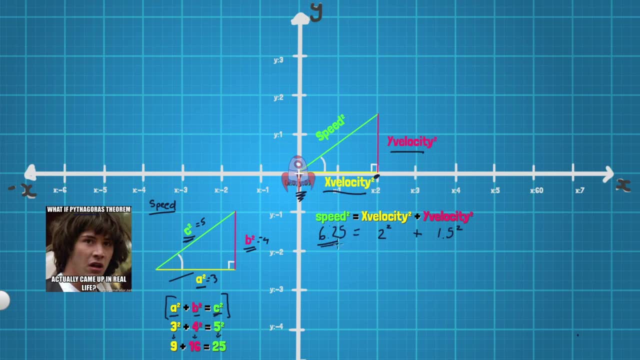 equal to six point two five. but there is an issue with this. 6.25 is actually the speed squared. that's what the two in the top right hand corner means. it means squared to find the actual speed. we need to take what's called the square root. here's a quick recap of the square root we're going to use. 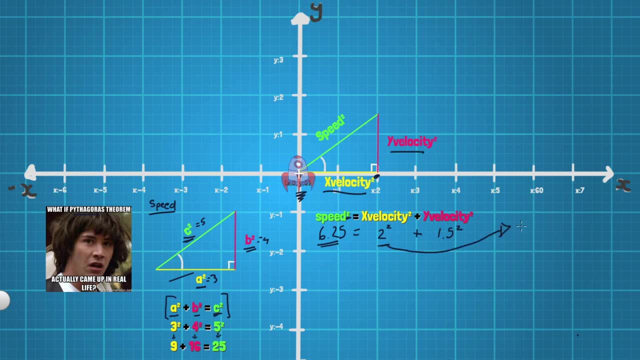 the x velocity, because that's a nice friendly number. the x velocity is two, and we know that 2 squared is just 2 times 2 and that's the same thing as 4.. so if we wanted to find what the square root is, the square root is signified by this little symbol here. and if we put four, 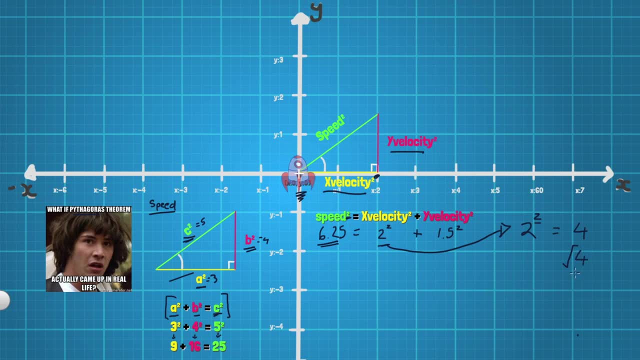 in there. we just want to know what number times itself is equal to the number inside the square root. so what number times itself is equal to 4? well, that's actually 2.. so 2 is equal to the square root of 4. Let's just do one more example: 3 squared, You know that, as 9, 3 times 3. 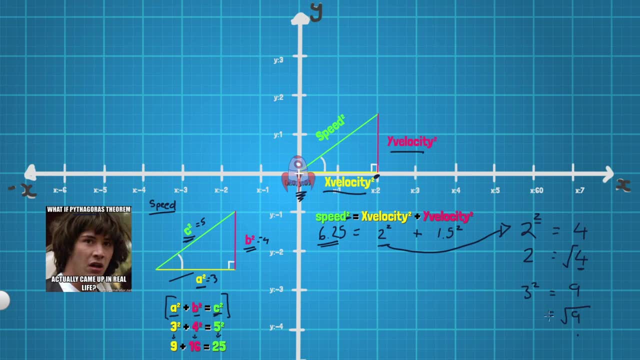 So the square root of 9 is going to be: that's right, It's going to be 3. so to find our speed, We want to find what the square root of 6.25 is, and the calculator tells me that that number is 2.5. 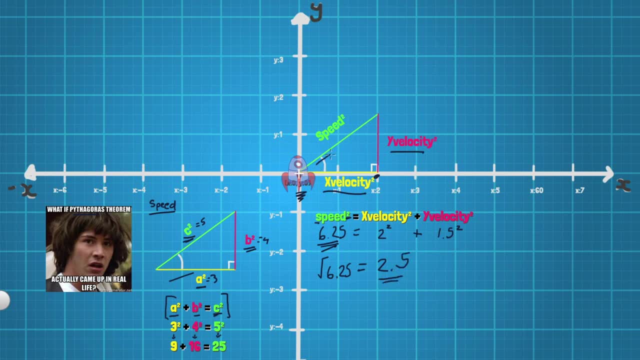 So 2.5 is our speed, and our speed is just the length of the hypotenuse. So our speed here is 2.5. So we can just slightly modify our formula and turn it into: speed is equal to the square root Of the x velocity squared plus the y velocity squared. 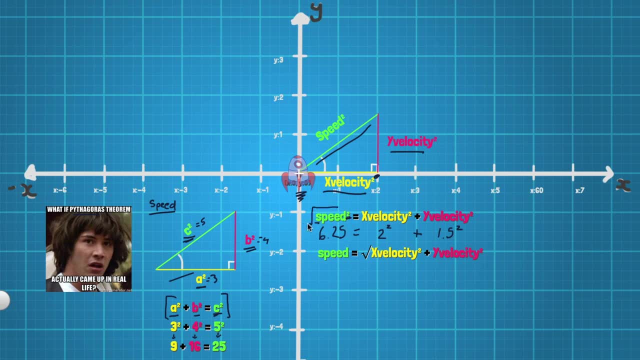 What we've done to get rid of the square here is: take the square root of speed. whatever we do to one side, We need to do to the other side, So that's where this square root comes from. Okay, you've been super patient And we're just about to get into scratch. 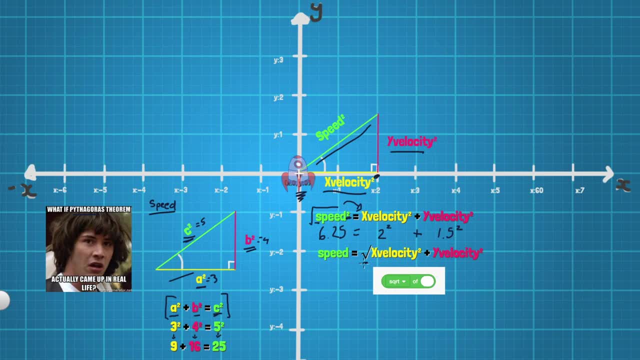 I just want to show you the block and scratch that you can use for the square root. So this square root symbol is represented by this scratch operator block and it's square root- SQ for square and RT for root- kind of looks like square. and now to tie this all neatly together: 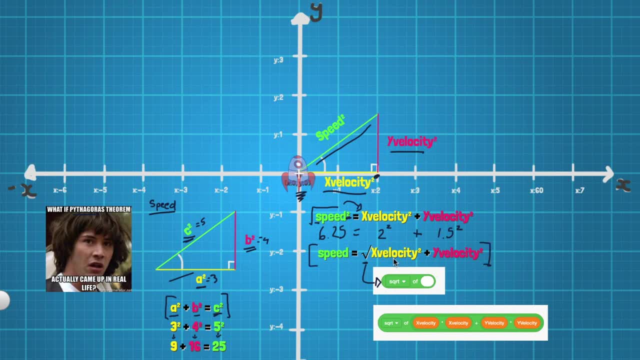 So this formula: here speed is equal To the square root of the velocity squared plus y velocity squared. Well, we can represent that in scratch by creating a variable called speed, and we just set speed to the square root of x velocity times X velocity plus y velocity times y velocity. Let's go do that across the scratch. 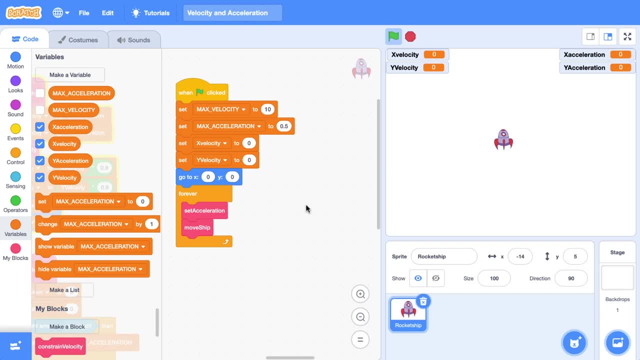 I'm just over here in scratch. Remember, grab the starter project if you don't have a copy of this already down in the description. Okay, we're gonna make a new variable. Yeah, we're gonna call it speed. after we move the ship, We're going to set speed. 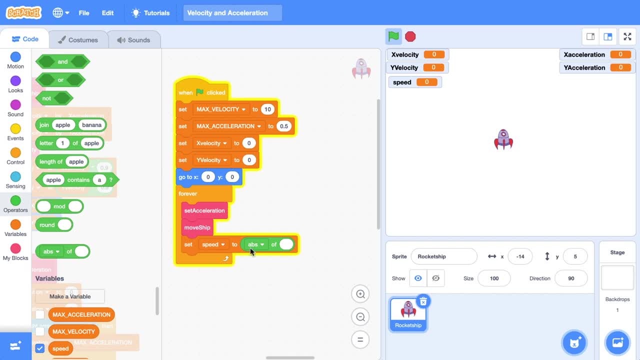 We're not going to set it to zero. We need to go grab that operator and change it from the absolute value To the squared value. Remember, we need to add together the x velocity squared and the y velocity squared, So we're gonna need some multiplication blocks.